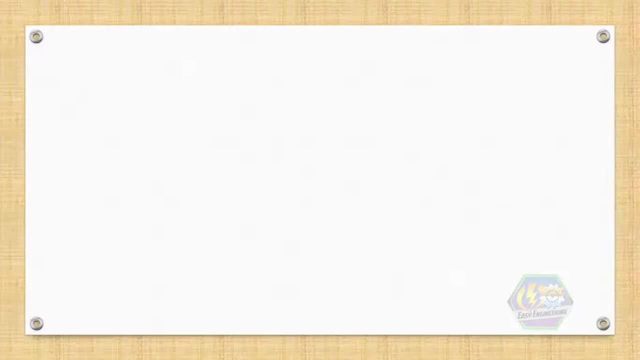 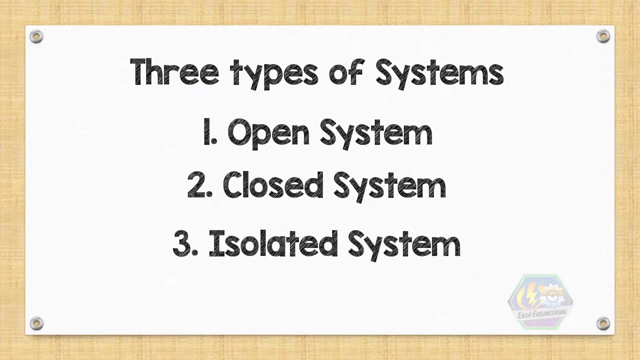 So let us move on to the second interesting part. I want you to know that there are 3 types away from our attention, namely open system, closed system and isolated system. To classify and identify what system are we looking at? time'� done the method of looking back to the history of a system, medicine, the interaction. 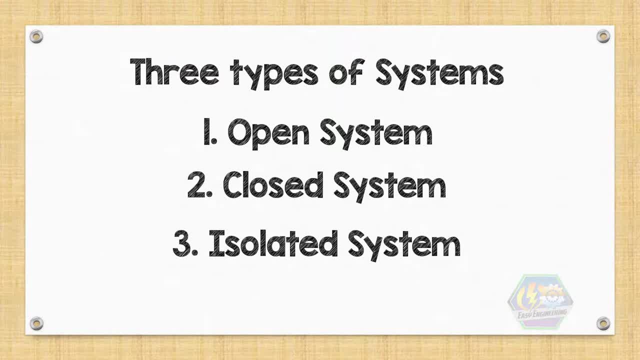 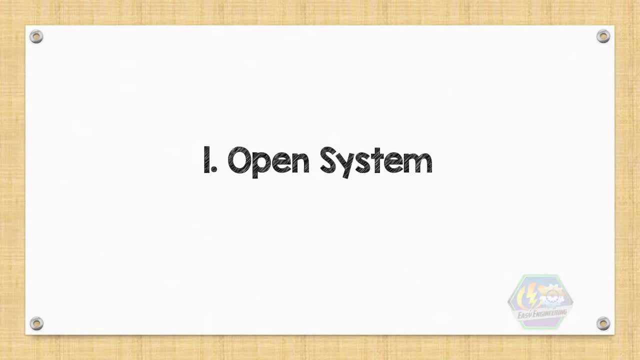 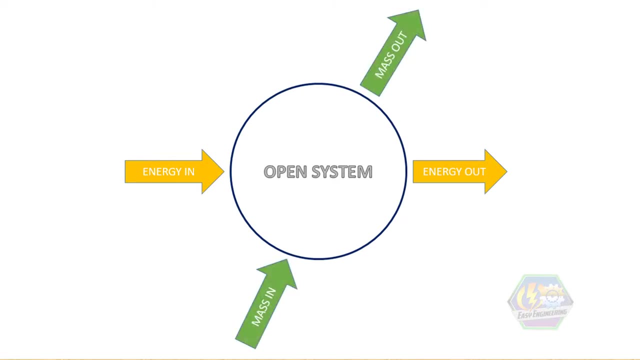 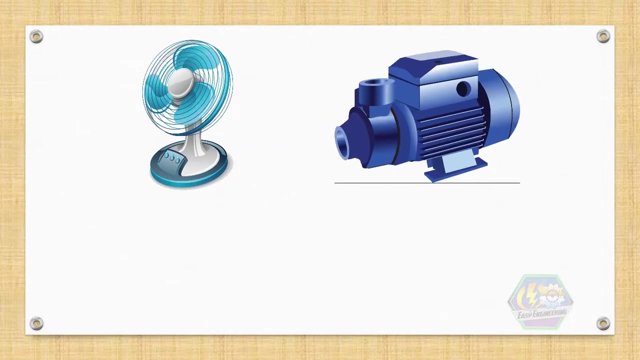 between a system and its surroundings that takes place across the boundary. so first let's talk about the open system. what interactions are in the open system? open system is a system which the boundary allows energy and mass to enter and exit the system. sample open systems are electric fan, pump, kettle and washing. 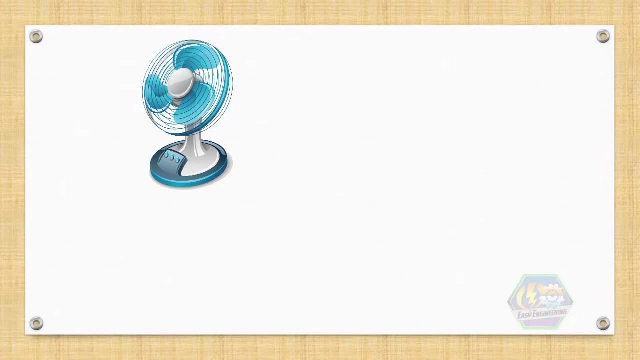 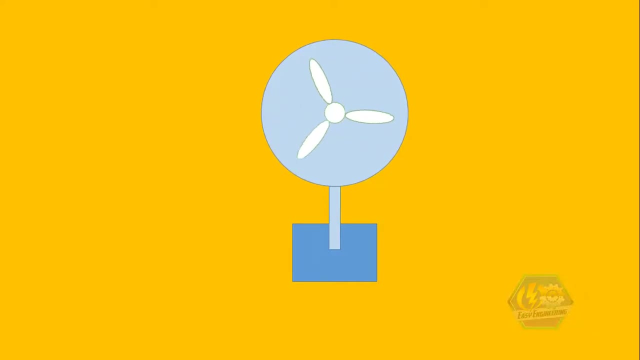 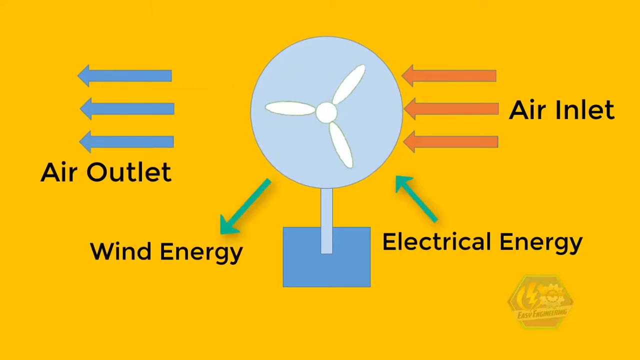 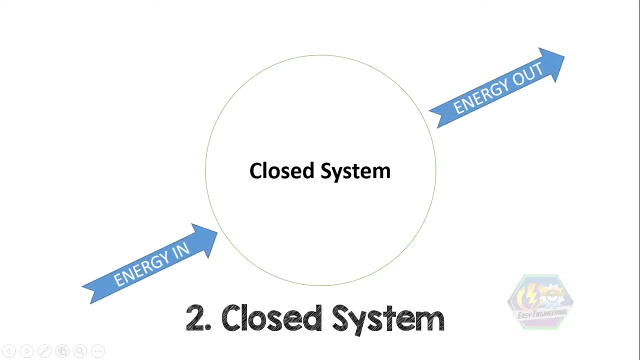 machine, considering it rains water. so let's take the electric fan for an illustration. energy enters the electric fan into its motor and when the blade of fan rotates, air gets drawn and discharged. very simple, right. let's proceed to the closed system in closed system. its boundary will only allow. 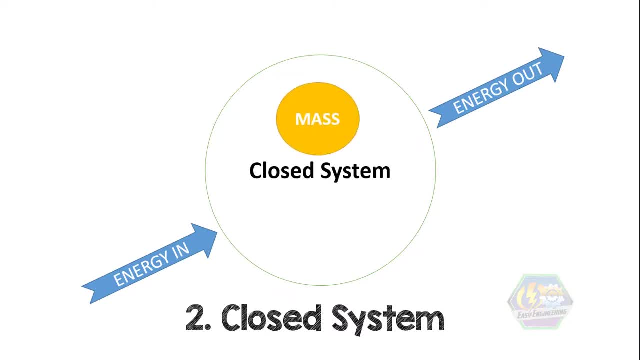 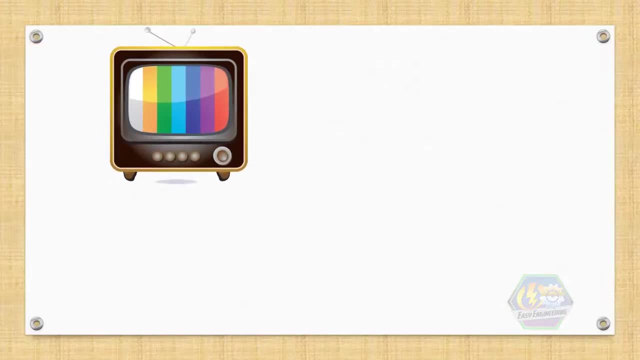 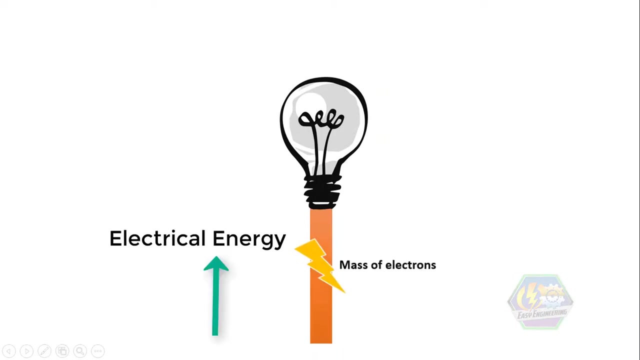 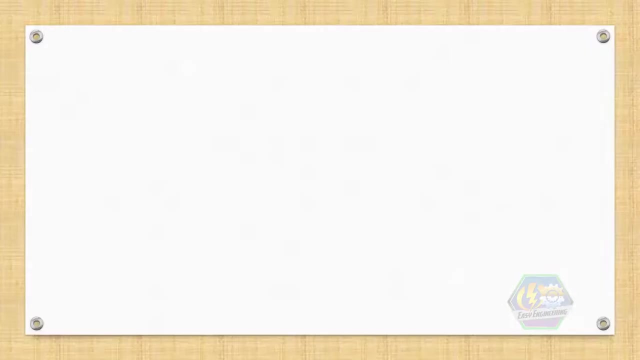 energy to pass and prevents the mass sample closed system are television, cell phone light bulb or the wheels on your car? for light bulb only. energy is allowed to enter and exit. the entering energy is the electrical energy and the exiting energy is the light and heat energy. the third system is the isolated system. isolated system. 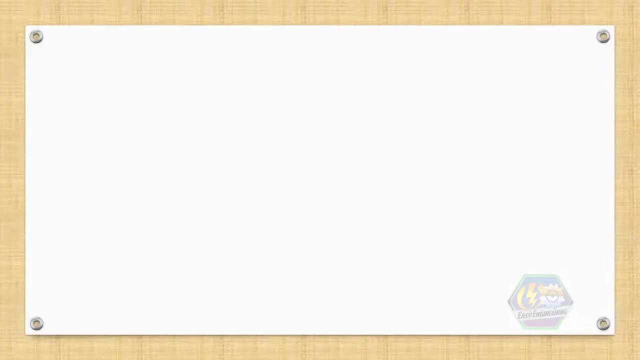 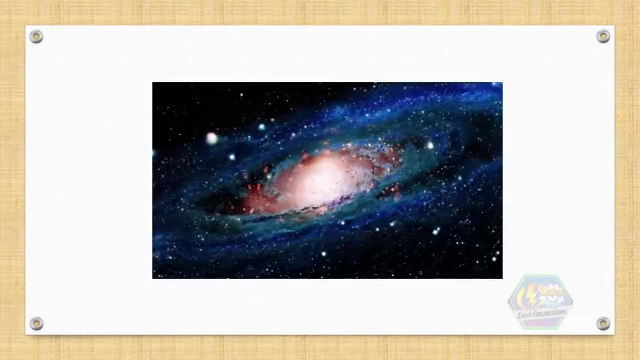 is a system which both the energy and mass are not allowed to pass in real world. the only sample system we can actually label as an isolated system is the universe itself. but for the sake of learning, we have systems that we call as an isolated system, as it acts like an isolated system for a finite period of 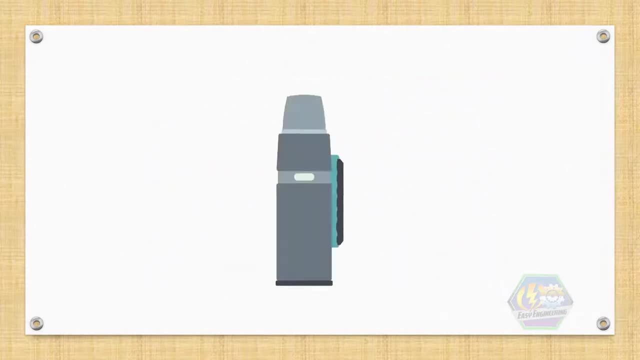 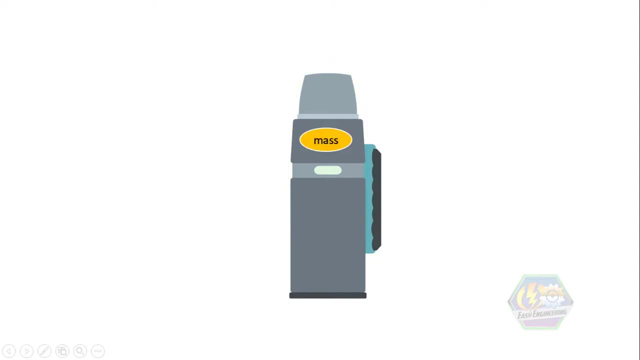 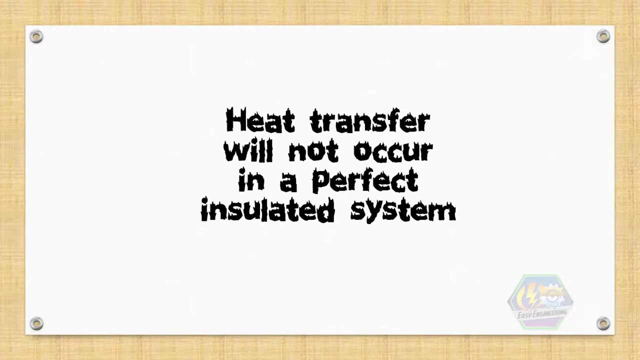 time. the best example that we can use is a thermos. assuming that the thermos contains a hot water which is perfectly insulated, there will be no way for the water to exit the container and hundred percent of its energy will be contained, as heat transfer will not occur for a perfectly insulated system. but, to remind,